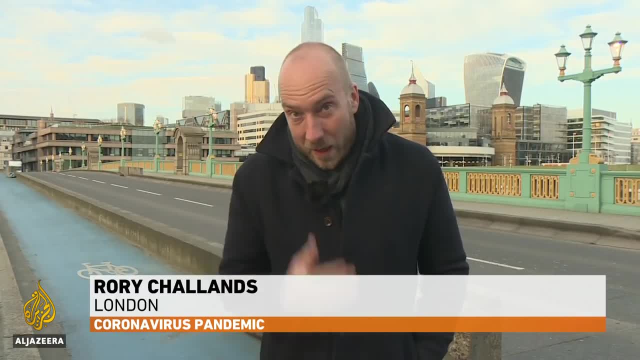 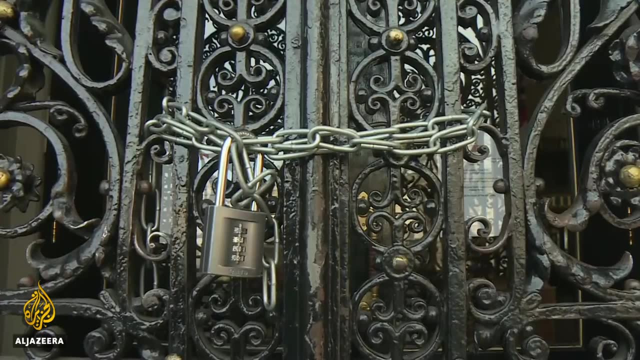 distancing measures the UK is following. Economically, culturally and socially. this is a country that has been transformed in just a few days By order of the governments. the UK is now pretty much closed: Pubs, cafes, restaurants, gyms. 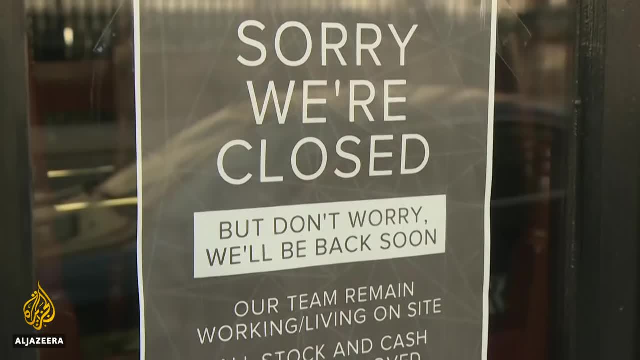 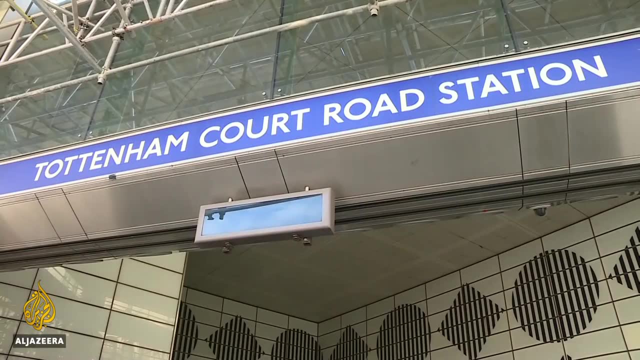 museums, nurseries, schools and universities all shut for the foreseeable future. The capital's buses are now closed. In addition to that, the city's public transport and metro system are empty. Don't use them unless your job is critical. people in London are being told This usually teeming metropolis. 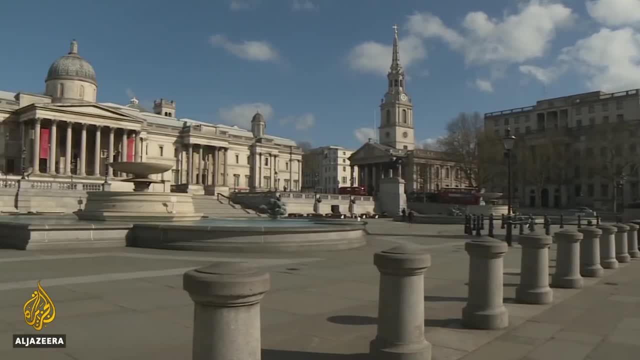 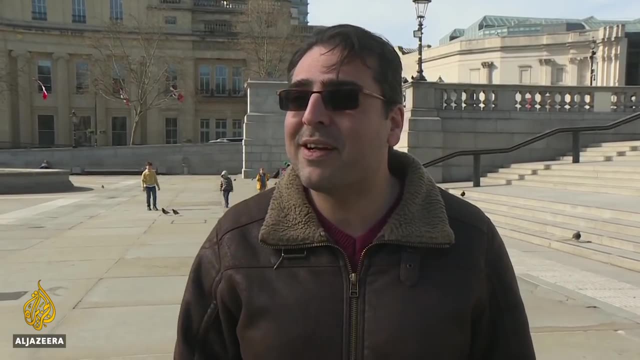 is quiet. I think it's good news. I think it's good news in terms of that they're looking after people that are losing out on their wages, the fact that they're stopping hopefully all spreading by closing down the restaurants- Yeah, I think they've done the right thing. 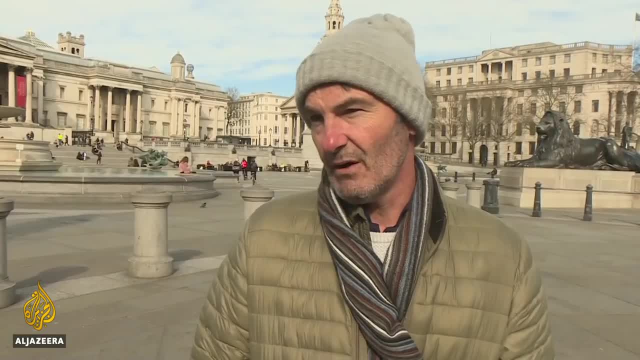 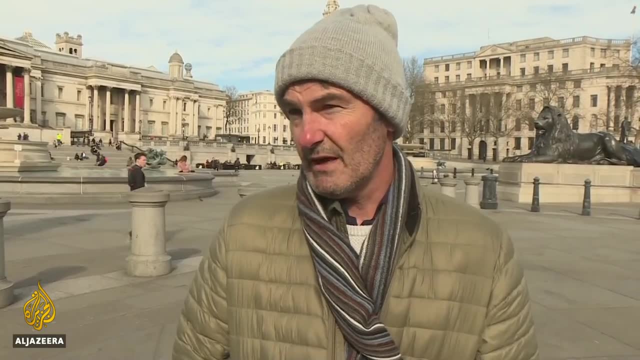 We went out last night for the last hurrah and sort of tipped up a little bit higher than we should have, I suppose. So just to sort of keep people going along. And yeah, it's sad for the smaller businesses but hopefully the government will kick in and sort of support. 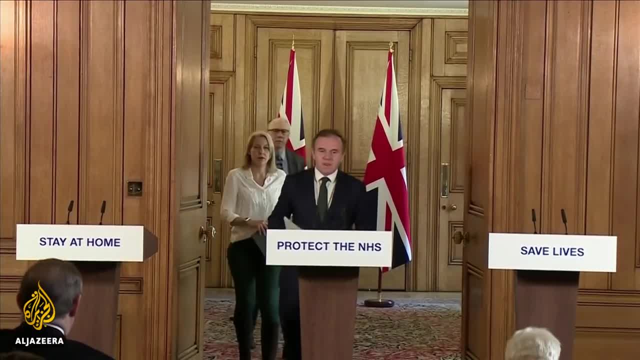 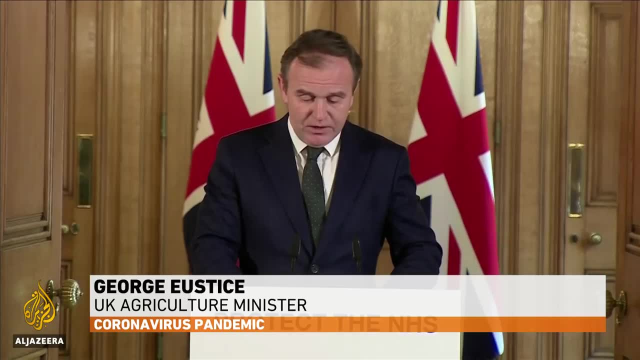 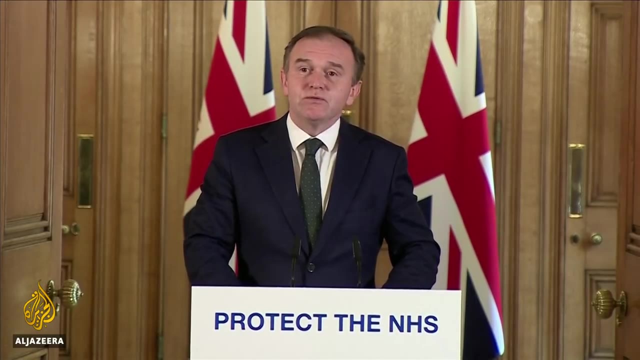 people along. The government is trying to stop a wave of panic buying that has stripped supermarket shelves bare this week. Be responsible when you shop and think of others. Buying more than you need means that others may be left without, And it is making life more difficult for those front-line workers. 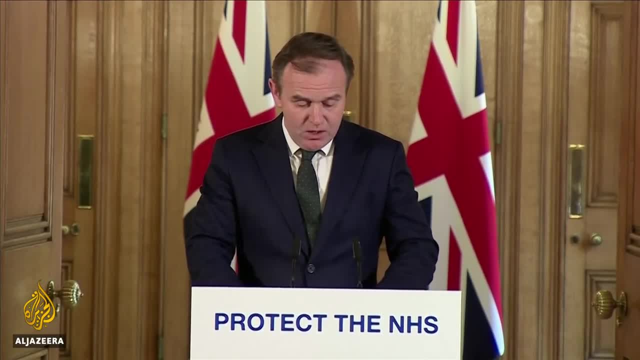 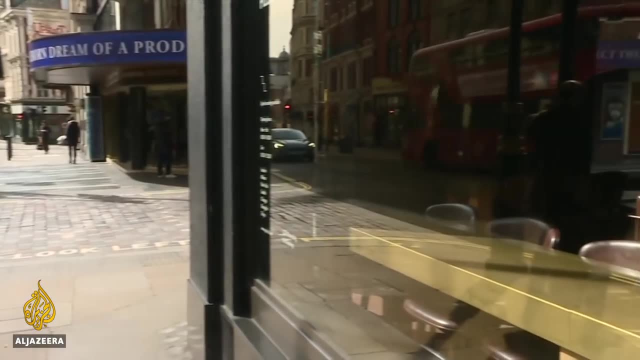 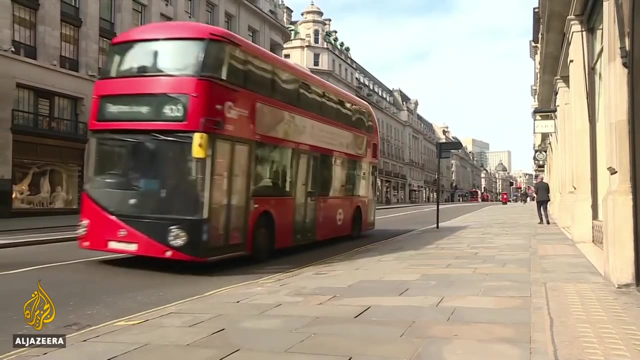 such as our doctors and nurses and NHS support staff, who are working so hard to make sure that they're not left behind in such difficult circumstances. To prevent total collapse, the government will prop up businesses and guarantee 80 per cent of all wages. It's an unprecedented temporary nationalisation of the UK's economy. Rory Challens, Al Jazeera London. 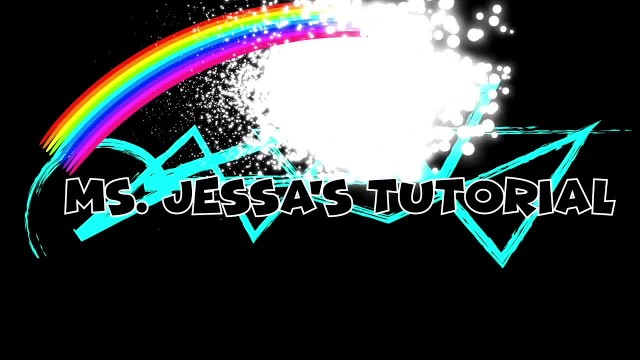 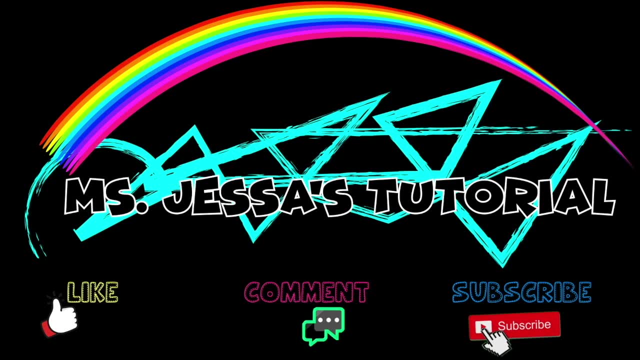 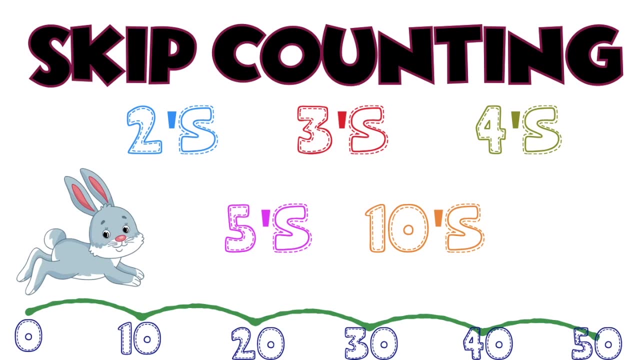 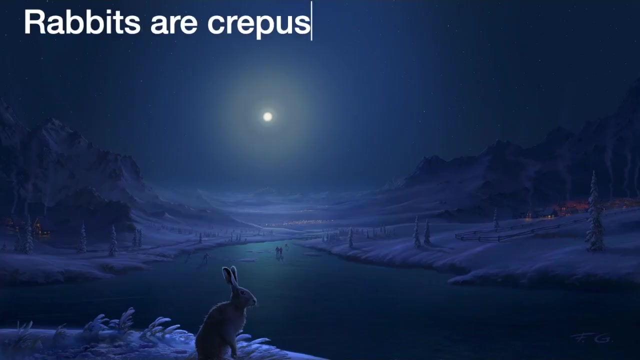 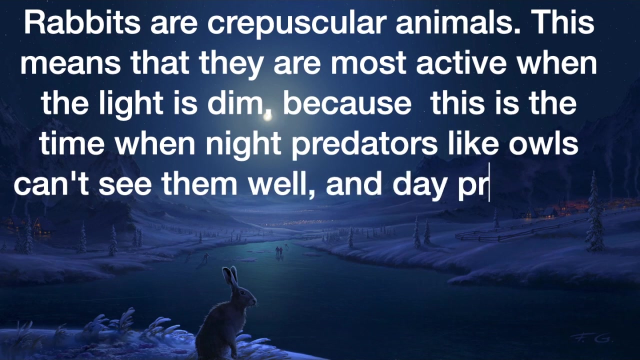 Today we're going to study skip counting by twos, threes, fours, fives and tens. Rabbits are crepuscular animals. This means that they are most active when the light is dim, because this is the time when night predators, like owls, can't see them well, and day predators.